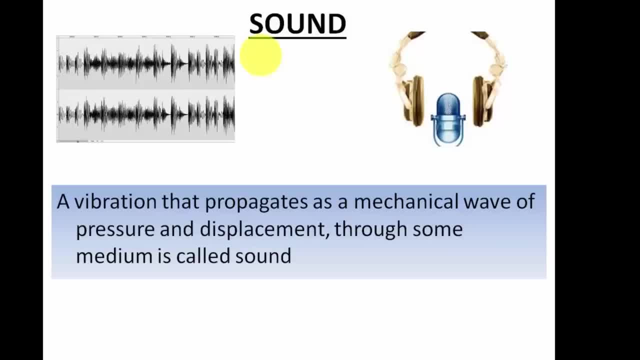 very annoying noise to another person, right, And this kind of rock music may be very, very hazardous for a particular person who doesn't like it, But for the to the other person it may sound very, very soothing And noise may differ And it may depend on the listener and the circumstances. So first, 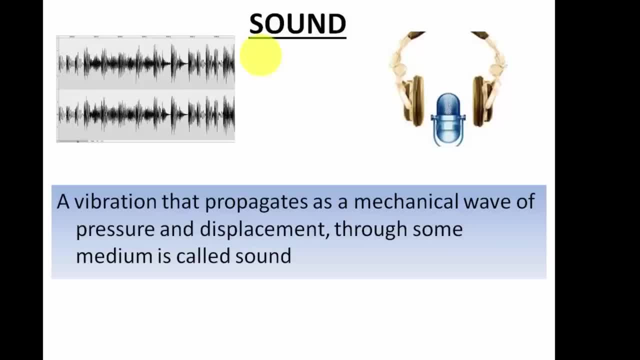 how do we define sound? Sound is a vibration that propagates as a mechanical wave of pressure, and displacement through some medium is called as sound. That is simple displacement of any wave. When a wave gets displayed, it produces, it is a kind of sound. What, on the other hand, 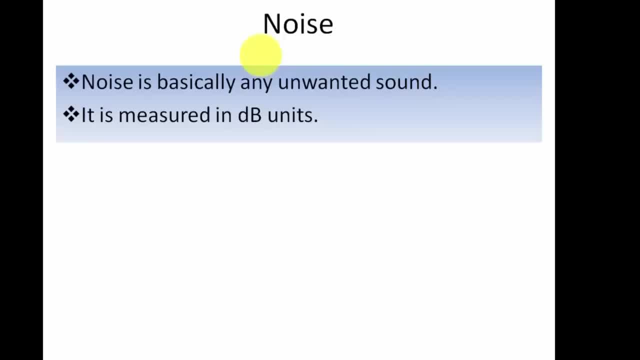 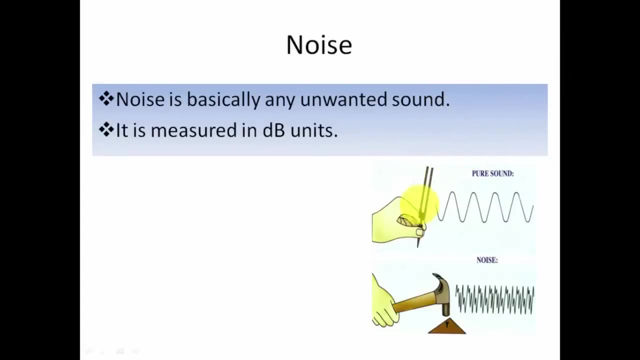 as we talked. Sound is noise pollution. Noise is basically, as I said is unwanted sound, Sound that we do not want, that we do not like, And this noise can be measured in decibels. So now, for example, if I take a tuning fork, so this is a tuning fork, and if I bang this tuning, 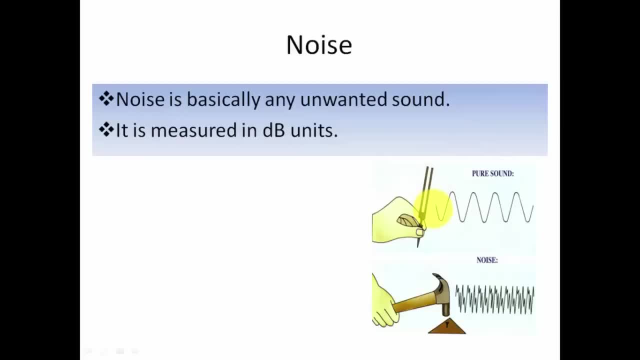 fork, I will get a sound. Now the vibrations will look something like this. The wave pattern will look something like this. It's a sine wave oscillation. On the other hand, if I take a hammer and if I nail a hammer, then the sound that is. 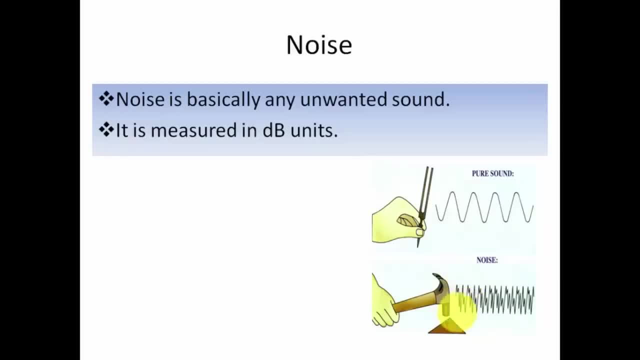 produced is not so soothing, and the kind of wave pattern which I get when I hammer a nail will be something like this, That is, it is so distorted, The wave pattern that is obtained while when I hammer a nail will be very, very distorted, right. So this is a kind of noise. 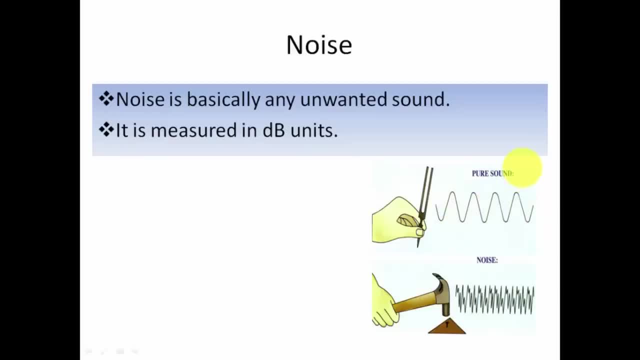 whereas this is a pure sound, Right. So that is the difference between a sound and a wave. Now let's see another, as we discussed previously also, that any rock music or a kind of music may sound very soothing to one person, But on the other hand, this person, he may feel that he is unnecessary, creating some. 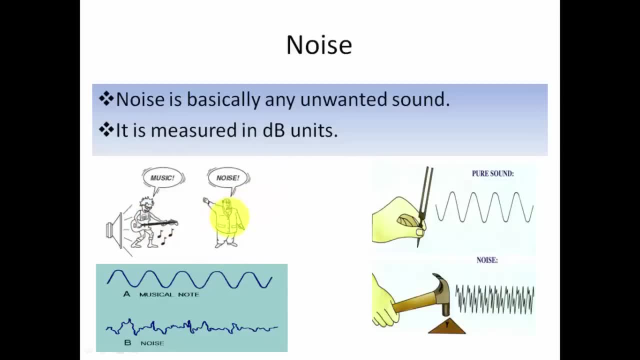 kind of noise because it is not at all interesting to this person. So, for example, a musical node, The wave pattern will look something like this: It's a sine wave oscillation again, whereas noise, the wave pattern of a noise, will be distorted like this. So that is the 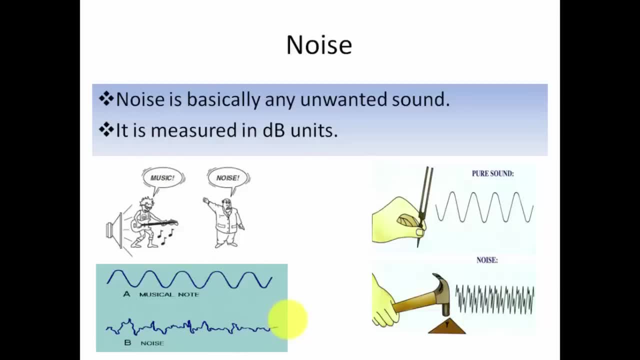 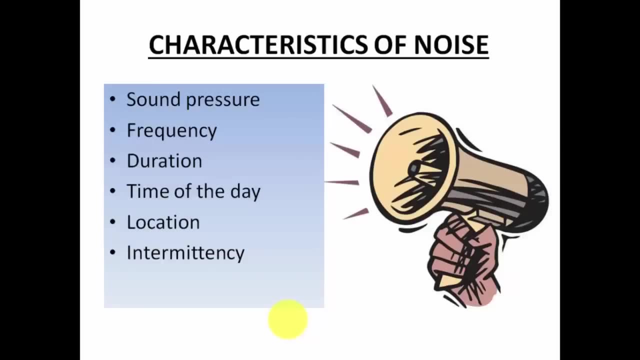 major difference between sound and noise. So now, what are the characteristics of noise? Noise may have various characteristics, and even sound will have these characteristics. For example, we have sound pressure. then is the frequency. And what is this frequency? Frequency is nothing, but it is a rate at which the sound is produced, The sound waves. 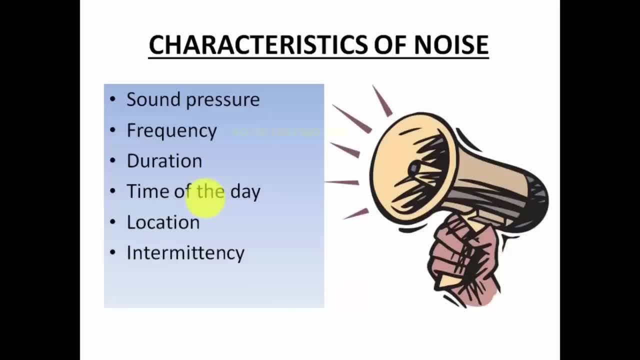 are produced. That is what is called as a frequency. Number of cycles of high and low pressure regions is what is known as the frequency. Next is duration, that is, duration of the noise or duration of sound, time of the day, location and intermittency. So these are the various characteristics of noise, or these can be the 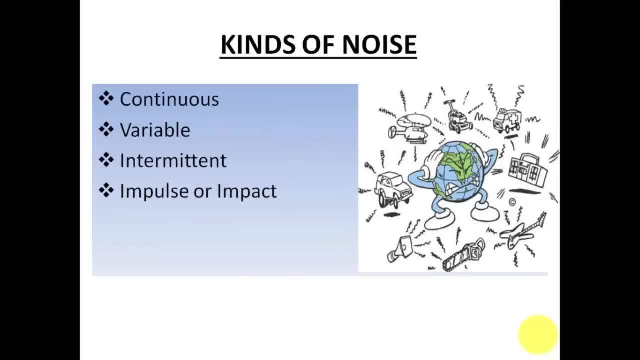 characteristic of sound also Right. So now we have various kinds of noise, and different kinds of noise are as shown. We have the continuous noise, variable noise, intermittent noise and impulse, or we can say impact noise. So we're going to talk about these different kinds of noises one by one. 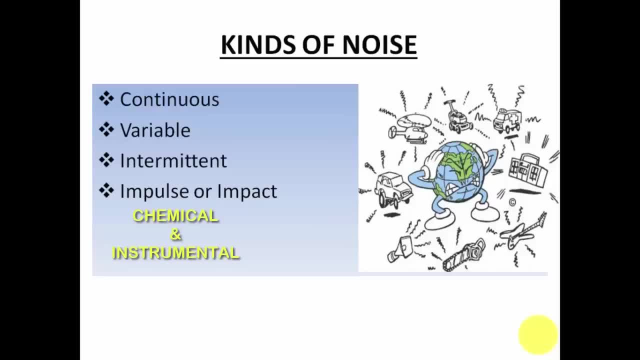 Of course there are other noises, like the chemical and the instrumental noise, but we were not going to talk about those noises in detail. But these are the four prominent kinds of noise That we'll talk about. So first kind of noise is the variable noise. What is variable noise? 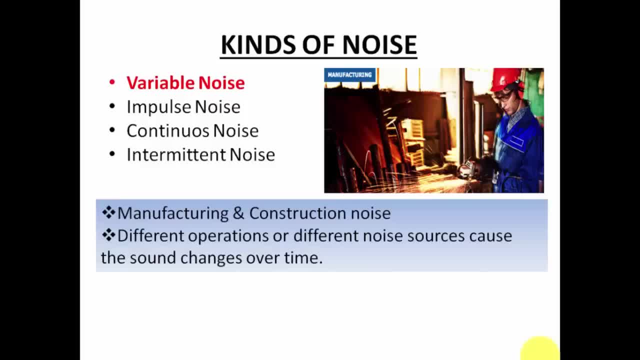 Variable noise is generally found in manufacturing and construction noise And because these are the operations which will generally have noises which will vary, the sounds and the noise will change at different intervals of time. Sometimes they will be high pitch, sometimes they will be low pitch sounds. So variable noises are produced in these kinds. 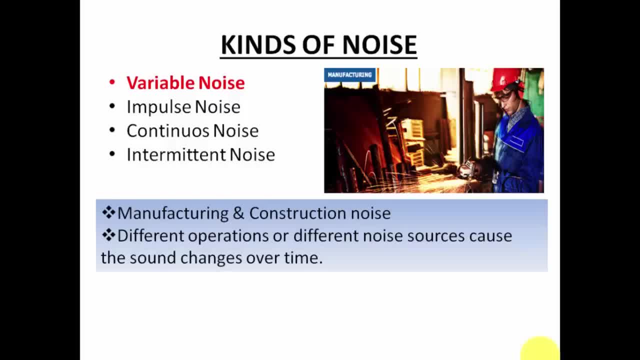 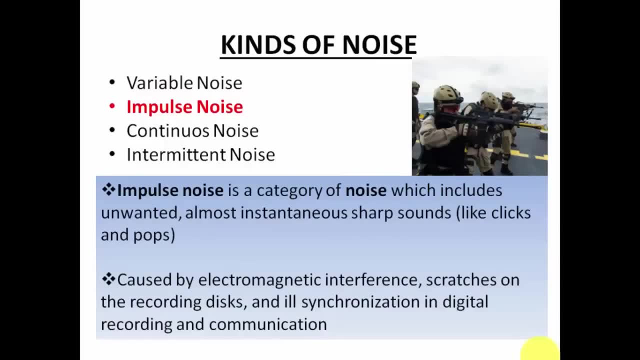 of manufacturing industries. So these are called as variable noise. Now, next is impulse noise. What is impulse noise? Impulse noise is a category of noise which includes unwanted, almost instantaneous, sharp noise like clicks and pops. So these are the gunshots, These 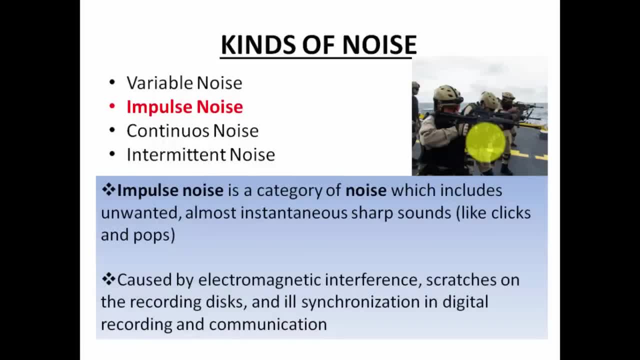 people are firing guns, So these are instant sound, just like a click or a shoot kind of, or pops, so these are called as impulse sounds. so noises of these kinds are usually caused by electromagnetic interference, scratches on the recording disc and some kind of ill synchronization in digital recording and communication. so these are the kinds of noise which are characterized. 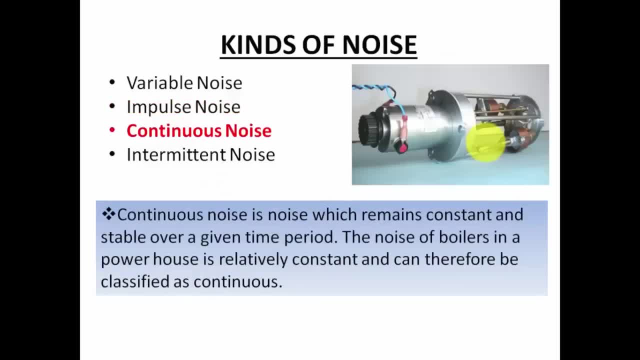 as the impulse noise. let's move on to discussing a continuous voice. what is continuous? by the name itself, it shows that these are some kind of noise which are continuously present, so those are called as continuous voice. for example, you see, this kind, this is a motor or a fan or some kind. 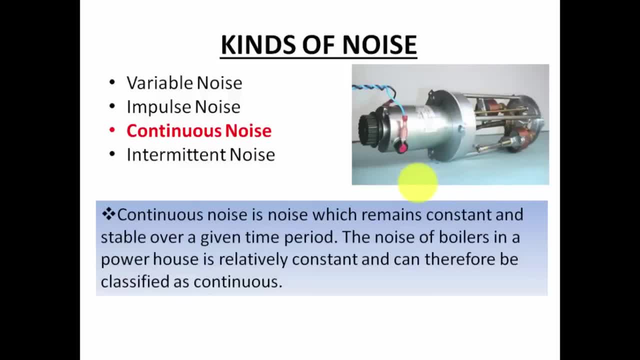 of boiler. so the kind of noise that is produced will will be constant. it will continue the same way for some time. so such noise are called as continuous noise. so continuous noise will remain constant and stable over a given time period. the noise of boiler in a powerhouse is relatively constant. 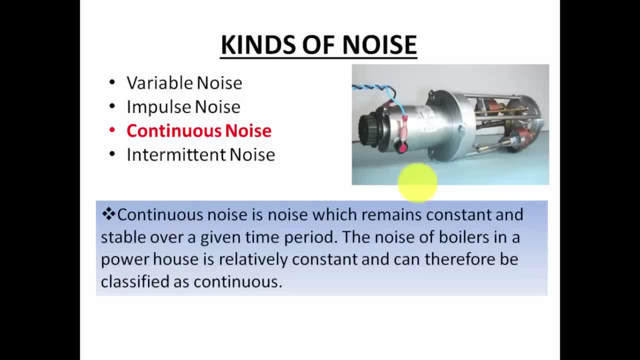 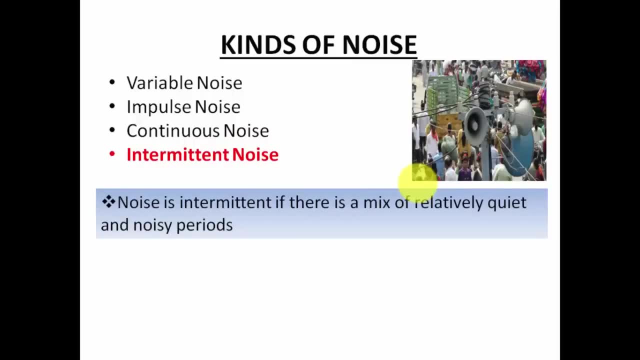 and can therefore be classified as continuous sounds. right next is intermittent noise. intermittent noise is a kind of noise where you will find a mix of relatively quiet and noisy periods, for example in a gathering where a lot of people have gathered, so you will find there are some people who are. 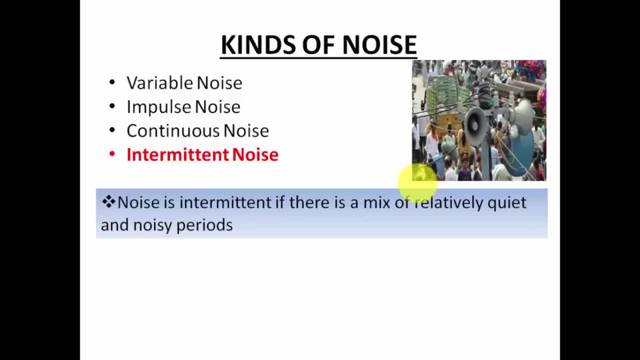 churning and there are some people who are talking very, very loudly, there are some who will be laughing, there are some who will just be quiet. so there are different intensity. the pitches will be different, so these are called as intermittent noise. sometimes there will be no noise, sometimes there will be high. 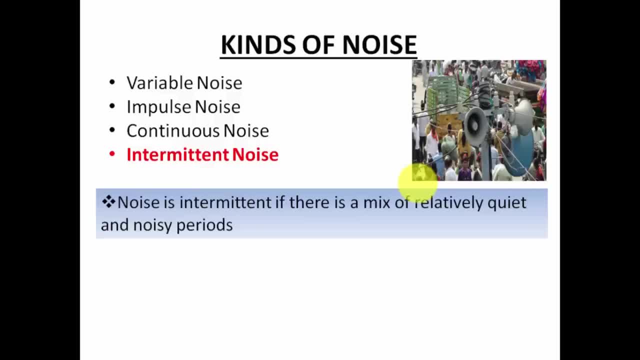 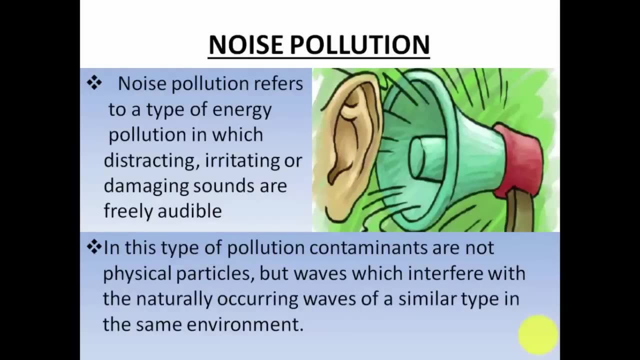 pitch noise, so those are intermittent noise. in between they will just keep popping, so such noise is known as intermittent noise. so these are the four very, very prominent kinds of noise. now that, and what are different types of noise? let's talk about noise pollution. what is noise pollution? noise pollution generally refers to a type of energy. 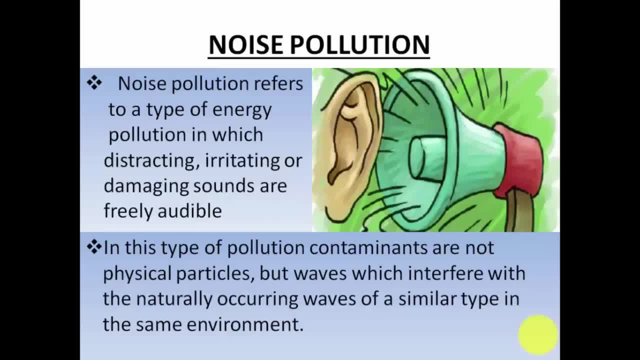 pollution in which distracting and irritating or damaging sounds are freely audible. right in this type of pollution, contaminants are not physical particles but waves which interfere with the naturally occurring waves of a similar type in the same environment. noise pollution, very simple words, is nothing but the emission of such a sound or such a noise which irritates us, which produce. 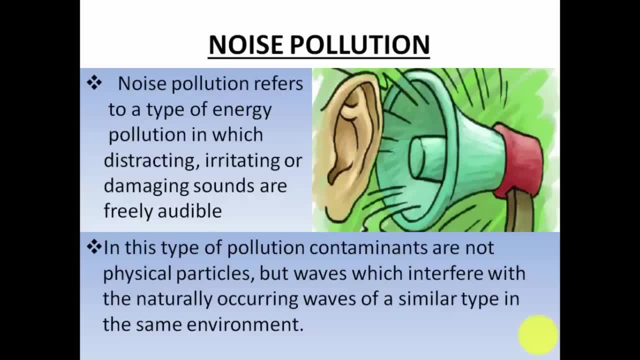 some kind of distracting noise is called as noise pollution. when there is a lot of sound which is unwanted, then this is called as noise pollution, and like when we talk about soil pollution or air pollution, then in in that case there are some physical particle that exist in water or in air. 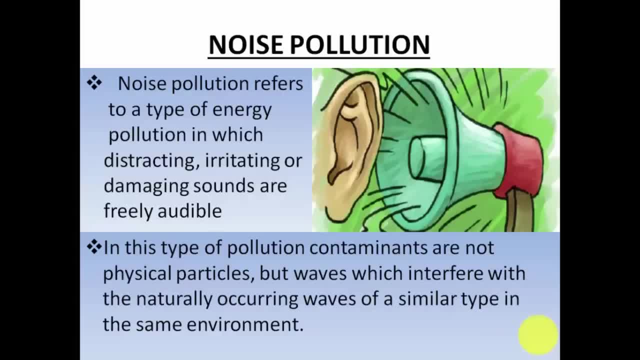 or in soil that pollutes, that contaminates environment. but in the case of noise pollution, there is no such physical particle existing, but it is just wave. it is just interference of two or three or more waves which produces this kind of distraction, noise, distracting sound, which we call a noise right. so this is what is known as. 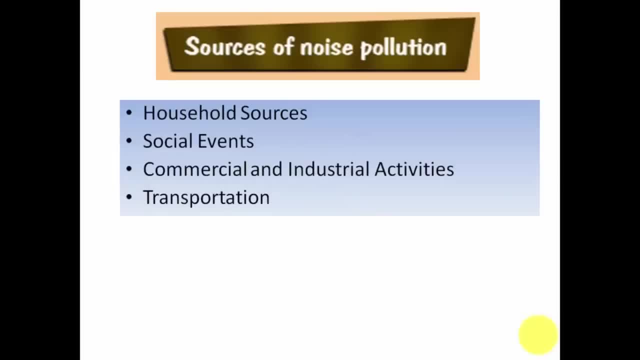 noise pollution. now, what are the sources of noise pollution? there are different sources of noise pollution. for example, we have the household sources. so by the name itself it suggests that household sources will consist of anything in the house which is creating some kind of distraction, some kind of noise. for 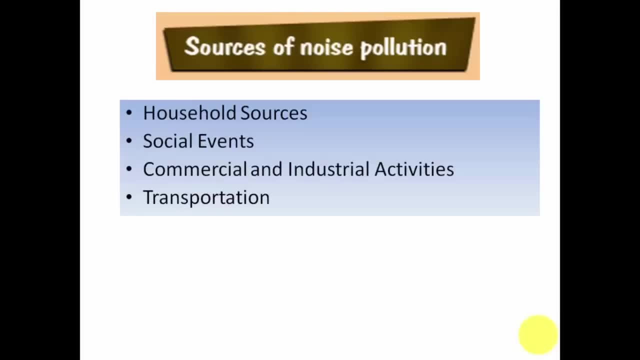 example the TV, the radio, the generator or the motors- if at all they are running in the house, or the washing machine right, or if the kids are playing in the park that is nearby in the locality, that is also household sources. if the neighbors are fighting, that is also household sources. next kind of sources: 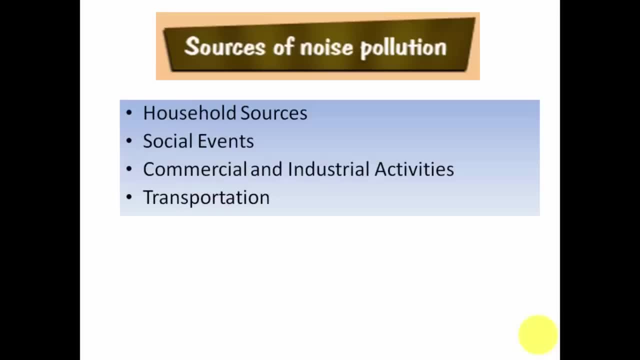 are social events, for example if there is a some community social gathering, or if there is an any public speeches which has been given by. you must have seen, these days the polish politicians keeps giving the speeches, so that is also some kind of social event which is happening, or any marriage which is taking place, or any. 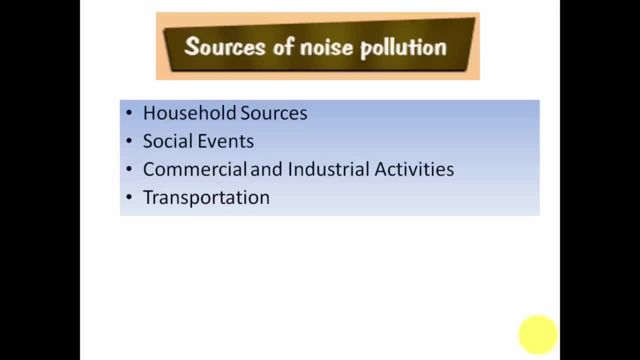 band which is passing by. so all these are social events which again produces some kind of noise, very loud noise, which are unwanted. right next is commercial and industrial activities. so these are like industries or the manufacturing industries or the production industries, some kind of some construction, if it is happening in the nearby locality, so that 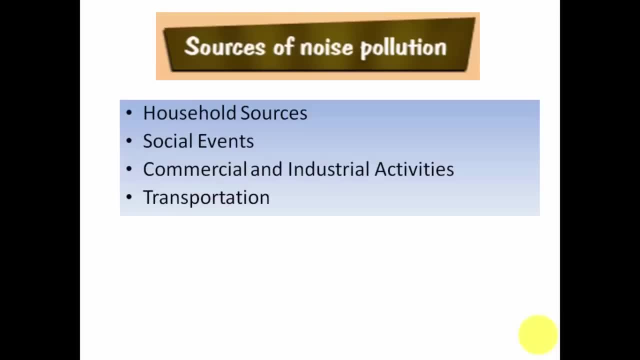 construction work again creates and produces lot of noise which is not required and unwanted. so these are the various kinds of sources from a commercial and industrial activities. then is a transportation to transportation. again, it is a major area- produces a lot of noise which are unwanted, for example the noise that is. 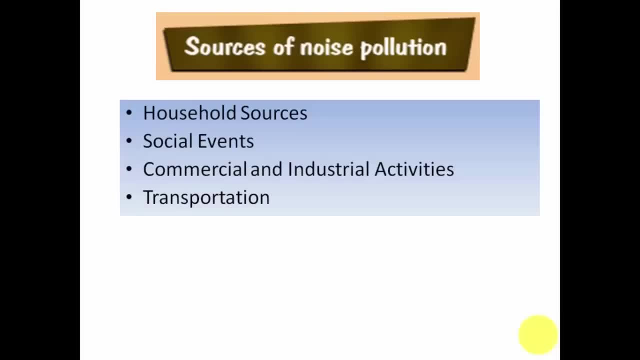 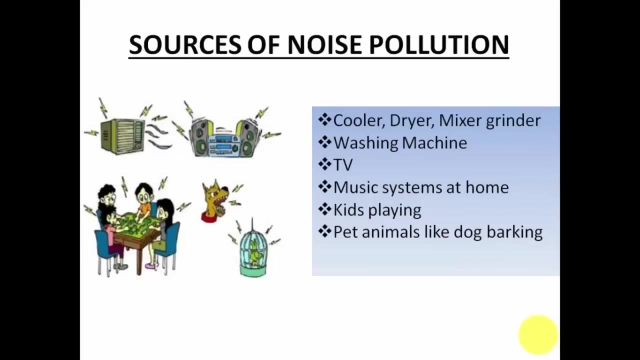 produced by various vehicles like auto, rickshaw, scooters, car, the horns of the cars, the aircrafts, the helicopters. so all these modes of transportation also produces lot of noise now. so first, these are the home, household sources which produce noise and, as I said, cooler, dryer, mixer and grinder, washing machine, TV. 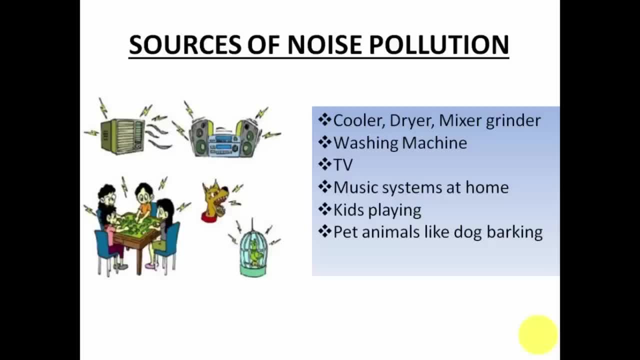 music systems at home, kids who are which are playing in the nearby locality. if there are any pets at home, they also produce a lot of sound. for example, the dogs are there, cats are there, so and the other pets, like the parrot, as you see here. so these are the various sources at home which produce noise. 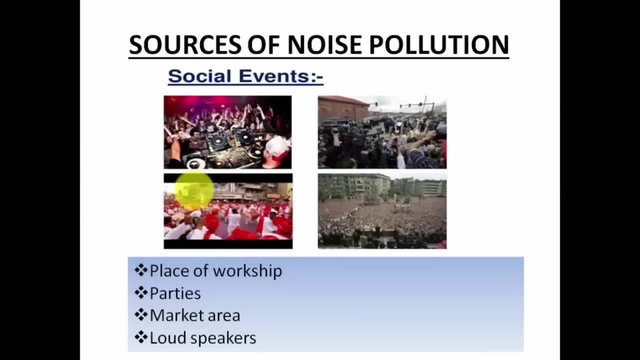 then the social event, as we just discussed, any kind of marriage which is taking place, any other kind of social events which are happening, or like pubs and restaurants. so the party area is a market area of any loudspeaker right, especially the place of workshop. generally, this is the area where we see. 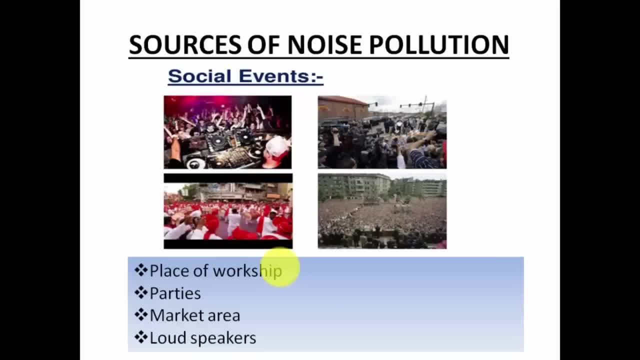 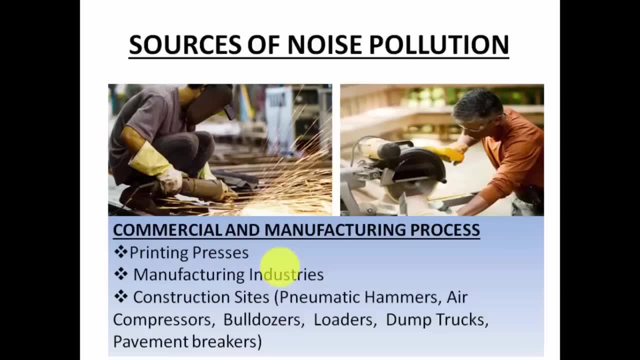 a lot of noise, you know being produced by people. so these are all social events which are producing noise. then we discussed about commercial and manufacturing process: printing press, manufacturing industries, construction sites, the noise that the bulldozers are producing loaders, the people who are working there. so all 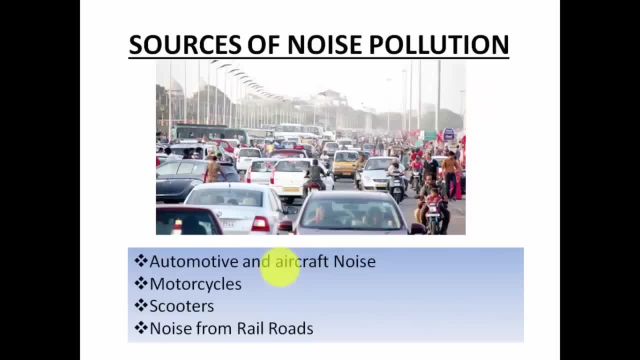 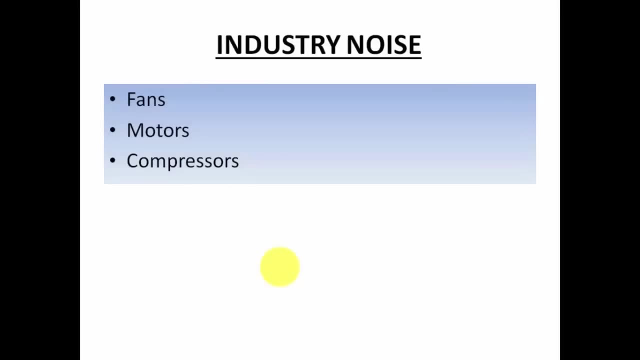 these are again commercial and manufacturing processes. then we talked about the noise pollution that is specially generated by the automobiles, the four wheelers, the motorcycles, scooters, and also noise from the rails. so these were the sources. again, we have few more sources apart from the four that we discussed, which are industry noises, that is, the fans motors. 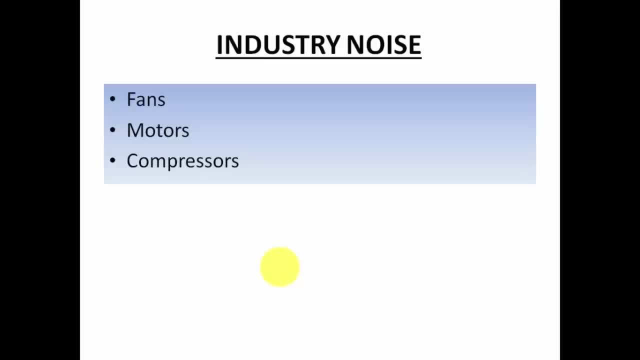 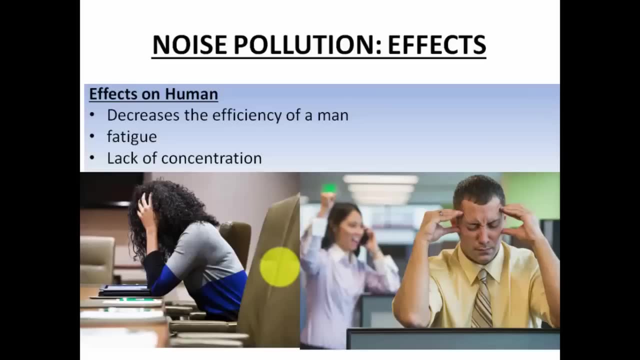 and compresses. these are major industry noises that are produced by these equipments. now let's discuss the effects of noise pollution. the effect is on the human health. noise that is produced by any kind of sources that we just discussed. it decreases the efficiency of man. and how does the 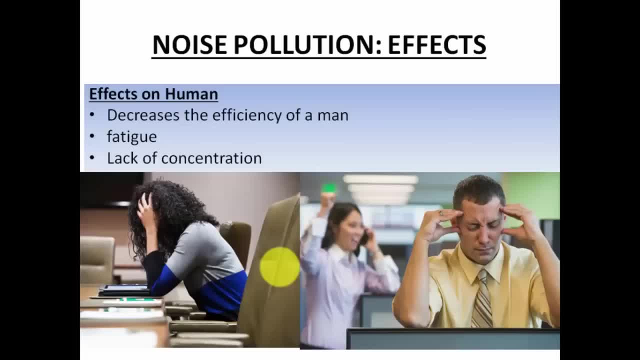 efficiency decreases. they are not able to concentrate on their work. they have headache the next day. if you can't sleep in the night, then you will have. you will have a sleepless night, you will not be able to take a rest and the next day morning you will not be fresh right. for example, you see in this picture the lady. 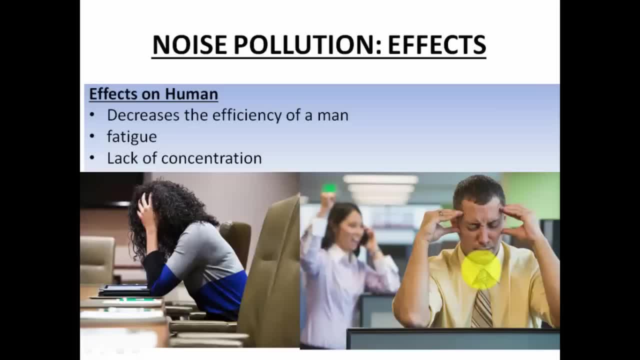 is talking very loudly. so this person, he is not able to concentrate and this will distract the person. so the distraction and decrease in the efficiency of any person can be of many times. first is distraction. secondly is that he is not able to concentrate because he could not sleep properly and he is fatigued. 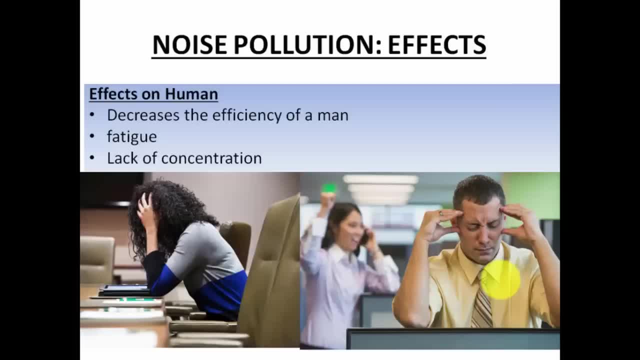 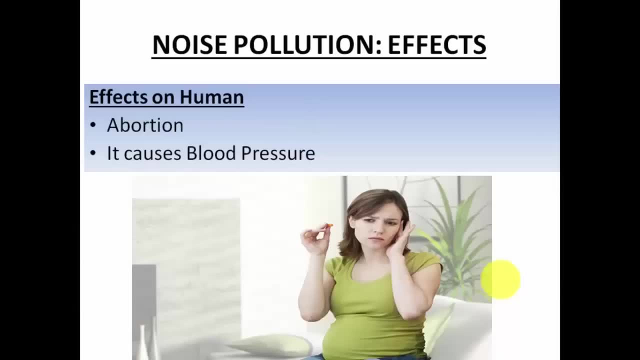 right. so fatigue is also a major effect of noise and lack of concentration, of course. next is abortion. a lot of noise can actually create and can lead to abortion of any lady who is carrying right. it also causes a lot of blood pressure problem. the blood pressure may may just become high or 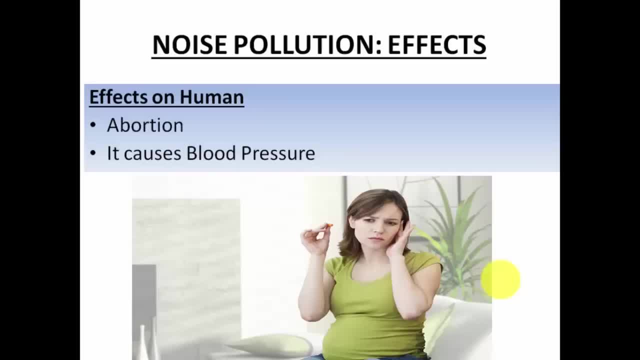 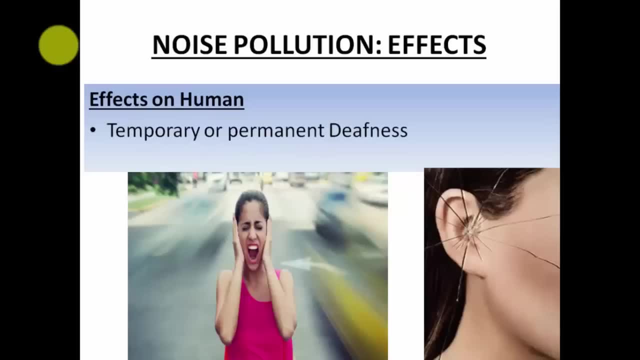 low. it may just fluctuate, so it is a loud noise is not good for any lady who is expecting, who is carrying a baby. other effects on human being is temporary or permanent deafness in case, sometimes because of loud noise, and especially the loud noise of the aircrafts. they may temporarily or 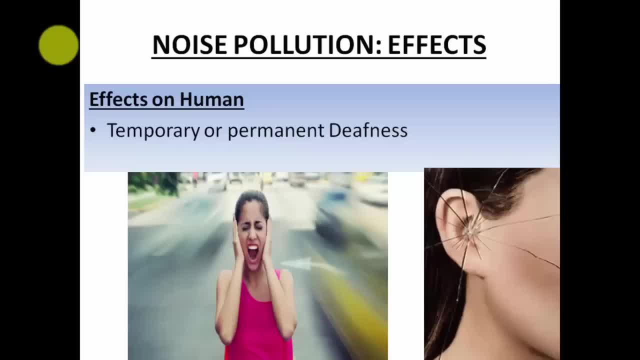 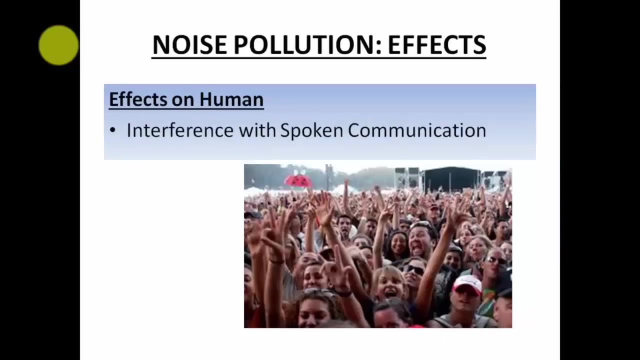 permanently create some kind of problems in our ears and the person may become over a long period of time. if a person is continuously exposed to high noise level then he may have problems with his hearing. he may become temporarily or permanently deaf. also, other effects are the interference with spoken 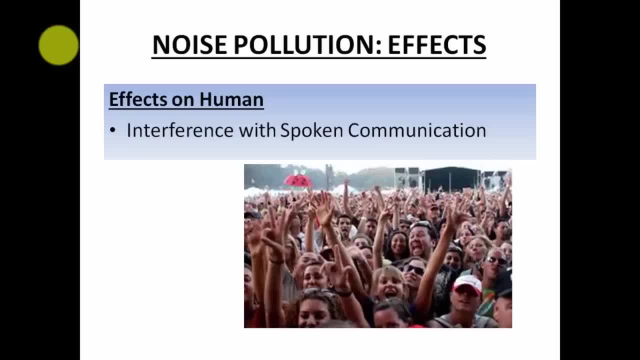 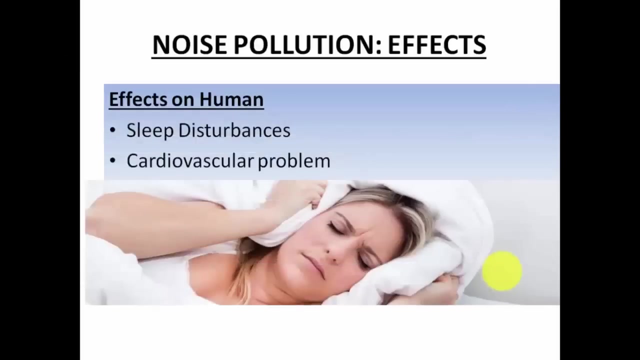 communication. like, as I said, if a person is speaking very loudly, then and if there is another group which is talking softly, so they will not be able to communicate effectively if there is any person in the vicinity who is talking loudly, because there will be interference. so interference is also a problem which is created because of noise, in case, let's 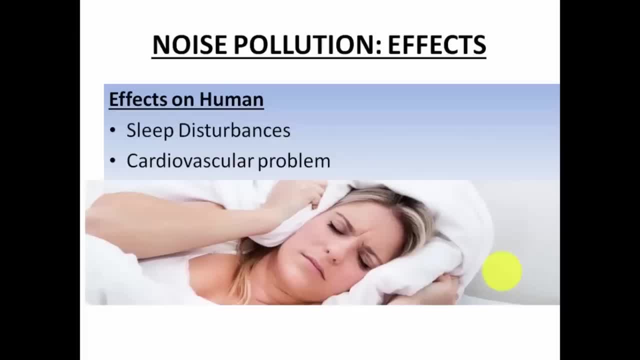 say that there is any social event or any gathering which is happening in a locality and if you try to sleep, then you will have disturbed sleep. you will not be able to sleep because of that loud noise of any marriage or any party going on in the vicinity. so in such case, 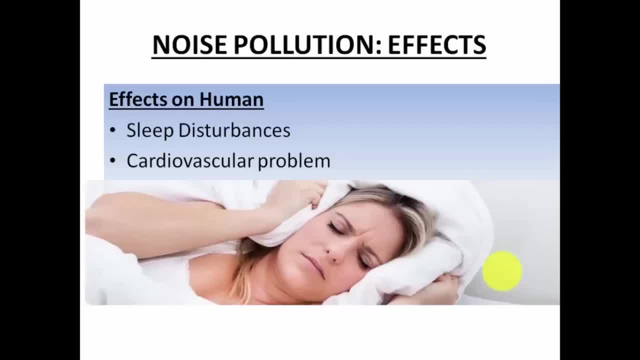 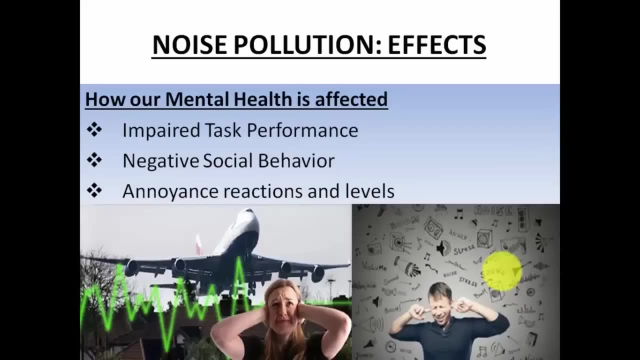 generally, a person will face a lot of sleep disturbance and this will lead to a lot of fatigue in the body and, over a period of time, a person may face some cardiovascular problem. okay, now how the noise pollution affects our mental health, because noise pollution generally leads to impaired task performance, also a 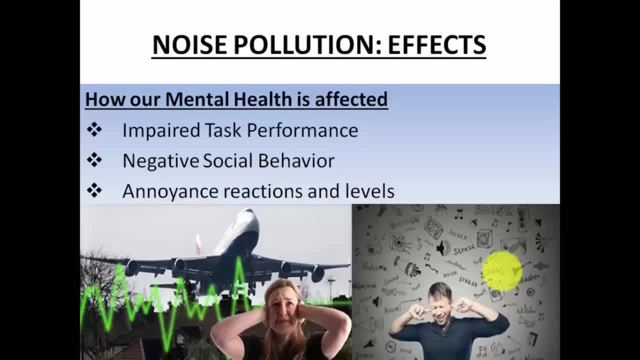 person may develop some kind of negative social behavior because, see, the next day he will be not fresh, then his behavior will be different, he will be irritated, he will have headache, and so this is the way he he will respond the next day to his colleagues and to his friends. the annoyance level will be high. the 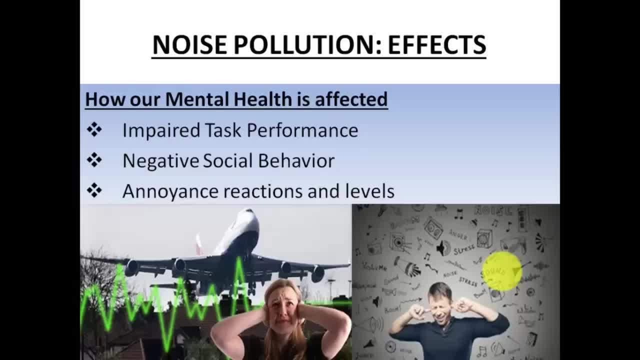 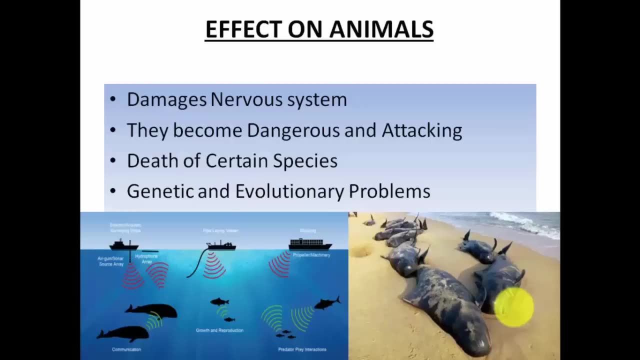 reactions will be very, very negative and ultimately, all these things combined together will affect a mental health of the person. now, even this noise pollution has very, very adverse effect on the health of the animals also, not just human beings, but also animals. and what are these harmful effects? first of all, the high level of noise, high intensity of noise. 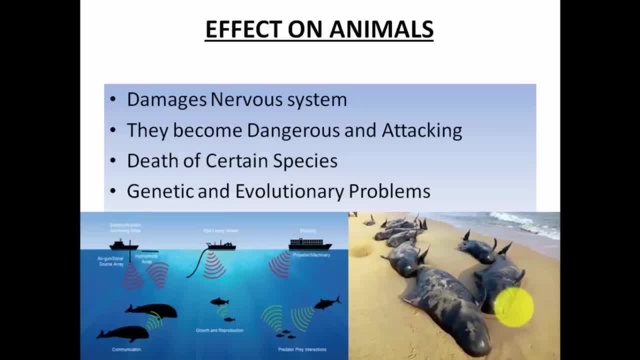 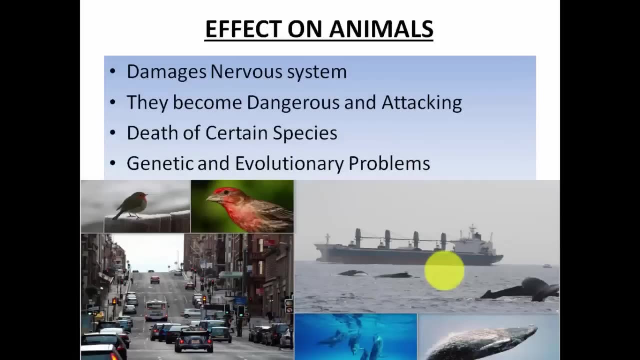 may affect, may damage the nervous system of the animals and the animals may lose control of its mind and these animals may become very, very dangerous and they may be attacking. also, a high level of noise may lead to death of some species. this also may have some genetic or some. 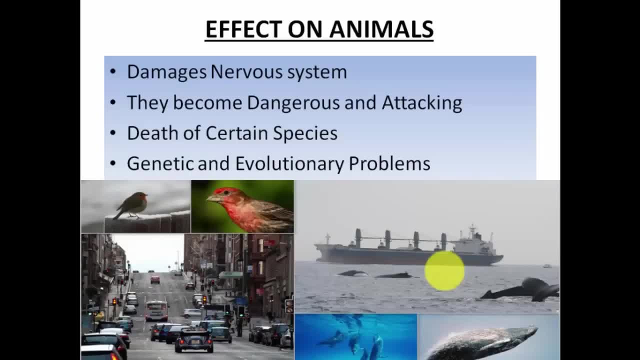 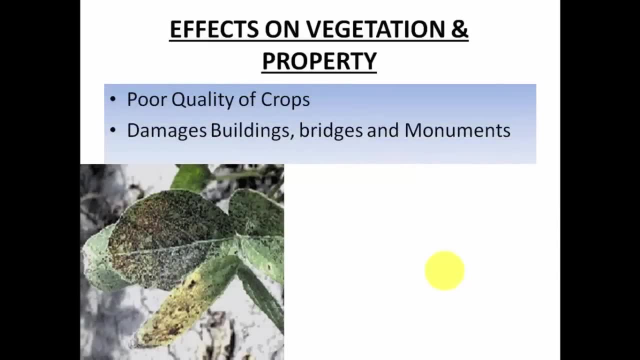 evolutionary problems in certain species. so these are few harmful effects on the body of the animals. now the effect on the vegetation and property. now, it is very well known to everybody that nowadays the plants are treated almost like human beings. right, they are also living. they also are sensitive to certain things, as man is sensitive to certain things. 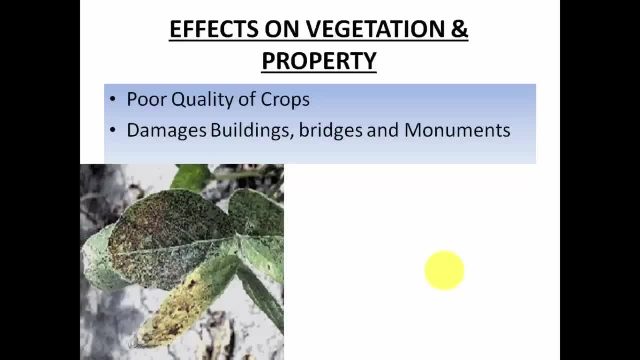 right, and even the plants need to be in some peaceful environment for their better growth and better quality of crop production- right. but this noise pollution actually causes poor quality of crop, even in a very, very pleasant atmosphere, even if there is proper rainfall, even is, even if there is proper. 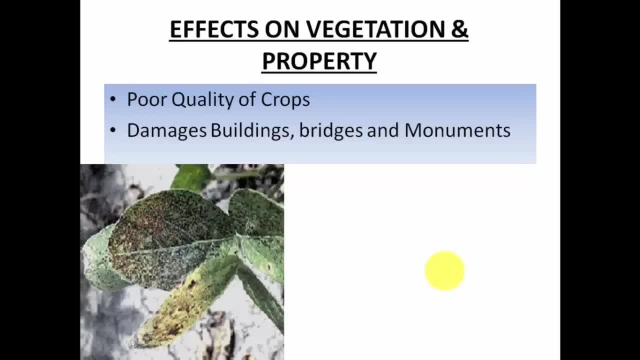 water supply, but if the noise levels are high then it will lead to poor quality of crops. now, when we talk about the property, noise, loud noise- is very dangerous to buildings, bridges, monuments. why is it dangerous? because it creates some kind of waves which struck the walls of these monuments and they 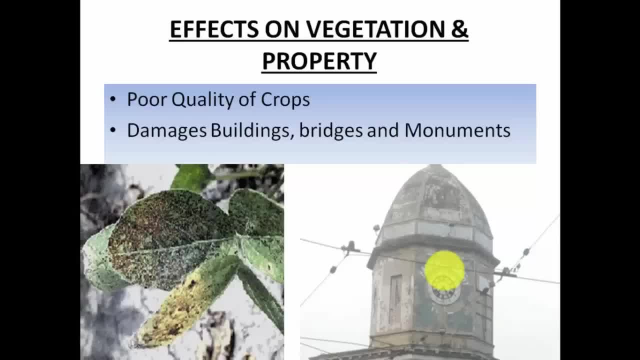 put the building into danger condition it weakens the building. basically it weakens the walls of the building. if the buildings are exposed to high levels of noise for a long period of time, then the walls of these monuments and these old buildings become weak. so these are some. 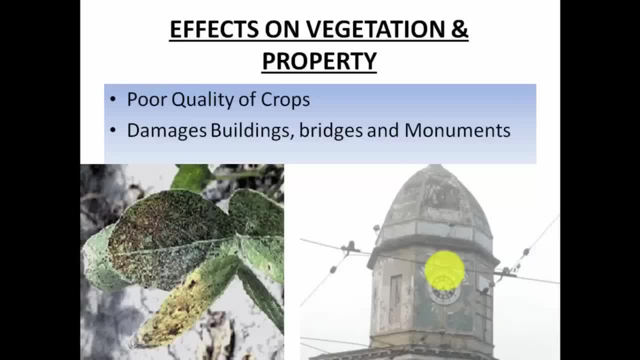 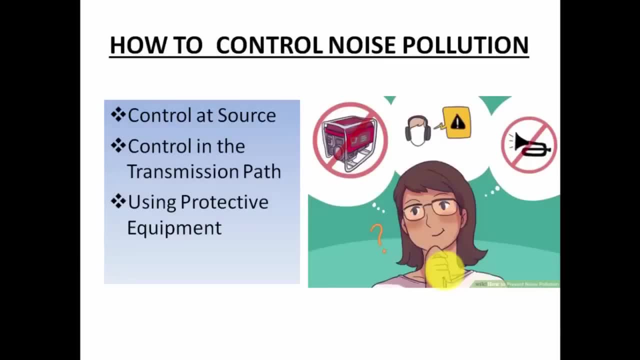 of the harmful effects of noise on vegetation and property. now, so what is the solution of the noise pollution? there are various methods and other measures by which we can control the noise pollution. for example, the first is we can control the noise at the source point only, that is, from 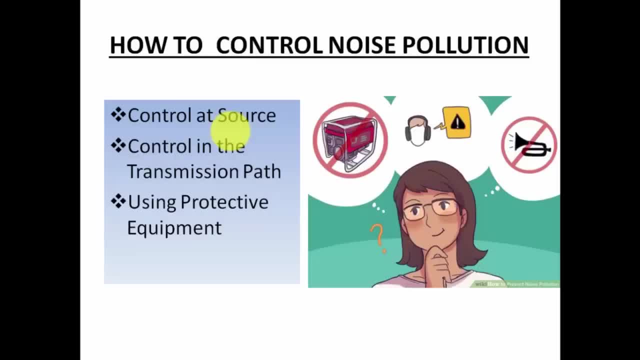 where it is originated, at that source itself. if we stop the noise, then the noise pollution can be controlled. the other thing is, if we control the transmission path, that is, the transmission path probably can be altered so that the noise pollution can be eliminated. the third method is: 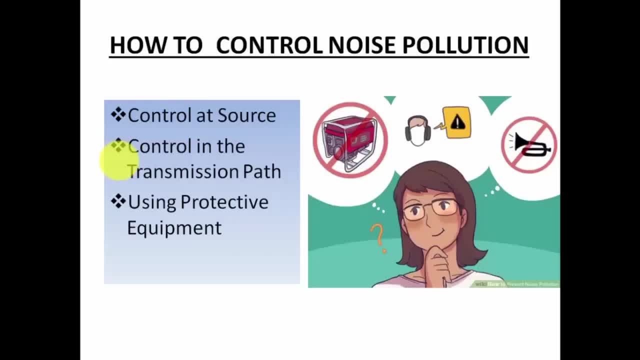 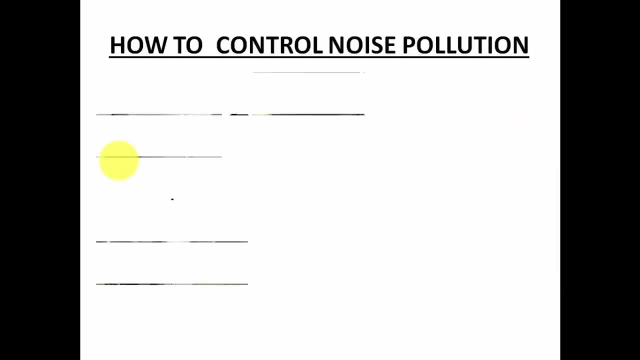 by using some kind of protected equipment, for example if we use ear defenders, so such equipments can be used so that the noise itself can be eliminated. so these are various measures by which the noise can be controlled. apart from these methods, the other methods that can be used is: 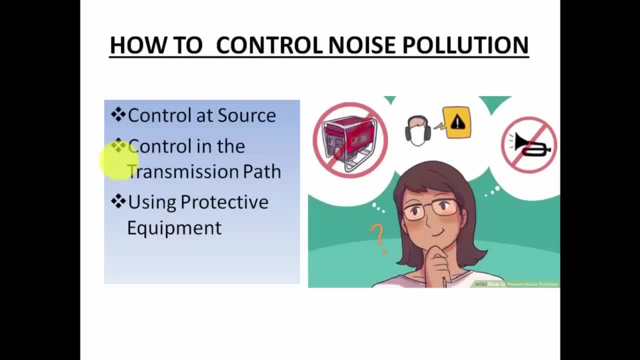 control over vibrations in case. see, sometimes the vibration are very, very smooth vibrations, which we use, and sometimes the vibrations are very, very unstable and they are very distorted, as we discussed. so if we control these vibrations properly, then maybe this noise pollution can be stopped. if we speak very slow, then again noise pollution can be controlled if we stop using such 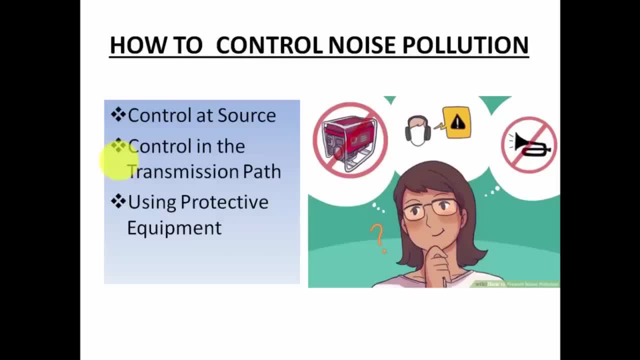 instrument which produce loud noise, again the noise pollution can be eliminated. and also, like we when we talked about the manufacturing and other industries, construction Industries, so in those Industries, if we use proper machinery which produces less noise, so again the noise pollution can be. so there are various methods by which either 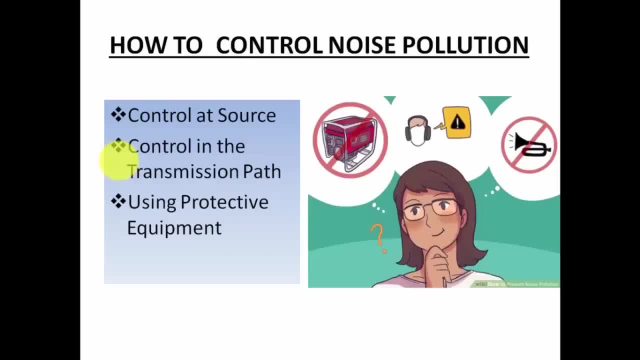 the noise can be reduced, or the noise can be eliminated, or the noise can be distracted. so there are various methods. now which method to choose? that depends upon the environment in which we are staying and in which we are facing such noise- high noise level, right. so for 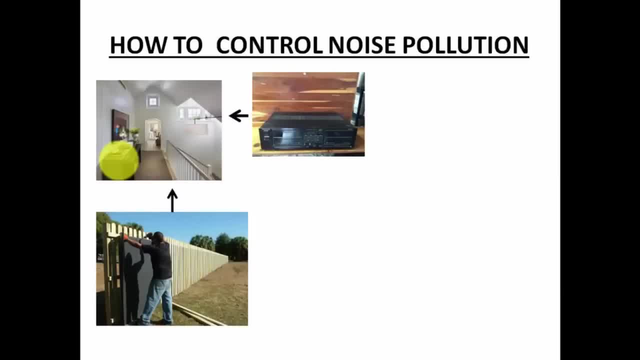 example, how can we control the noise, like if we talk about household noises? probably what can be done is that the amplifiers or the loudspeakers that we use or the music that we are playing- loud music that is being played in the houses- that can be stopped. any kind of construction work that is. 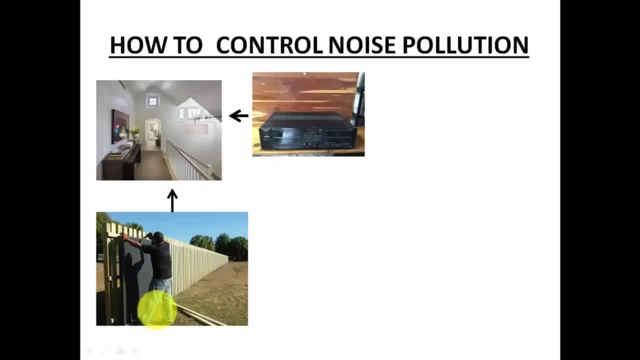 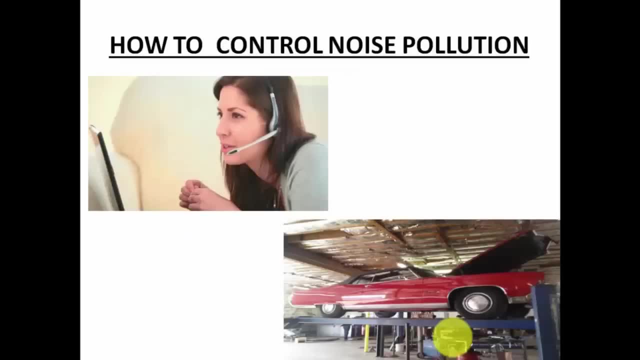 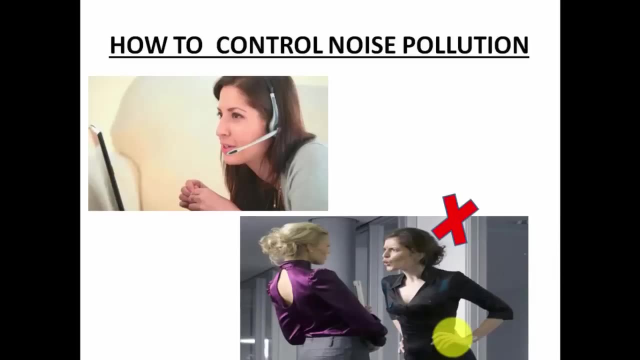 going on in the vicinity or in the gardens or by the neighbors. if we stop that, then again the noise level can be reduced. there are people who talk very loudly. so if we reduce the noise level again we can control noise pollution. there is any kind of fighting. so if we stop that again, 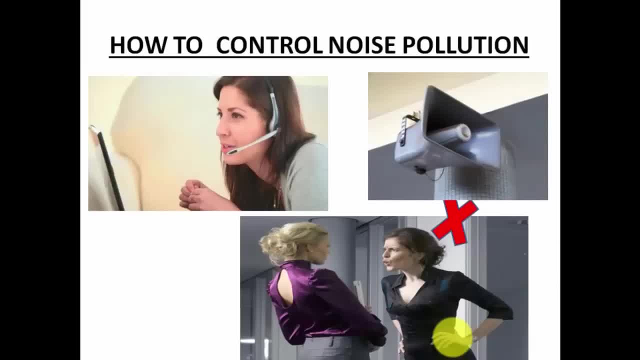 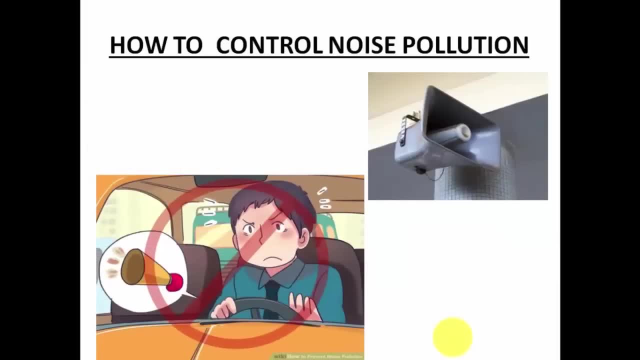 the noise can be controlled if the use of loudspeaker is reduced, that then again noise pollution can be controlled. another thing is that while traveling in our two-wheelers, in our four-wheelers, we should and must avoid unnecessary honking or unnecessary blowing of the horns of our 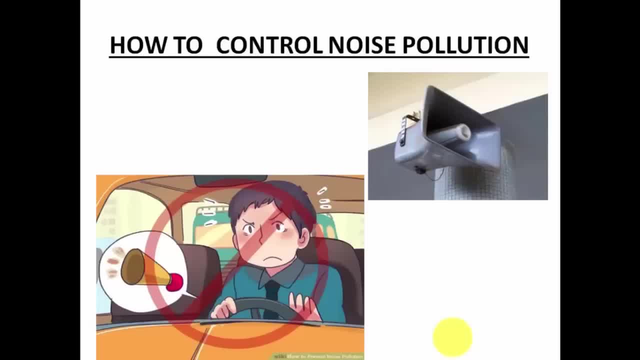 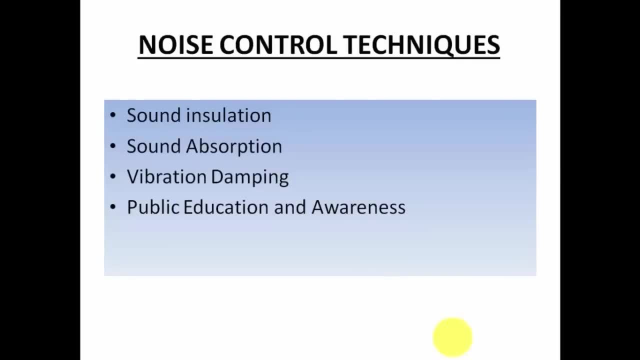 automobiles, and if this is done, then a large amount of noise pollution can be stopped. so these were the methods that we just discussed. these are the methods that we can do. we can start from our own, can do these small, small steps to avoid noise pollution, but otherwise there are professional 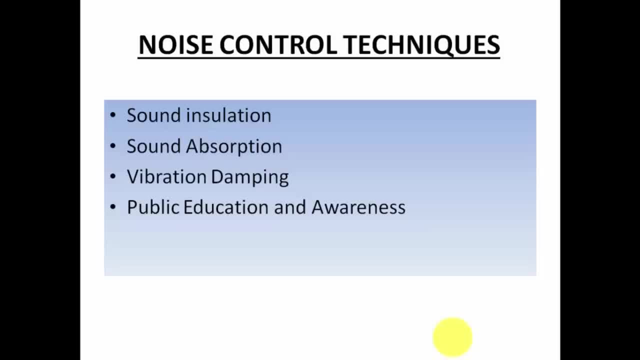 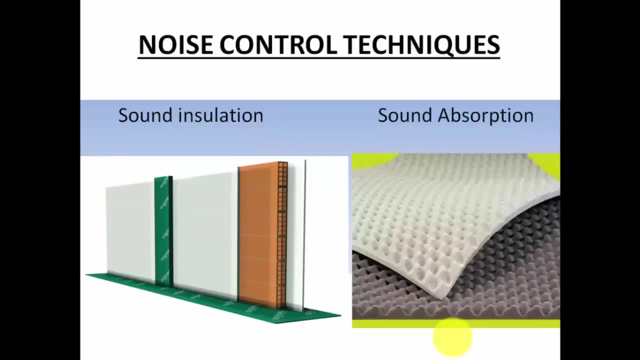 techniques by which the noise can be reduced or it can be eliminated, and those techniques are sound absorption, vibration damping, and public education and awareness. so let's talk about these techniques first: sound insulation and sound absorption. now, sound insulation is all about slowing or stopping the sound waves by physically blocking their travel from one room to another room. 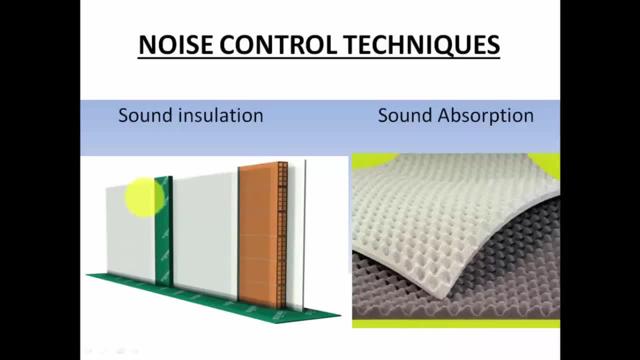 and how do we do so? now, as you see here, these are some kind of sheets that you see here. so these sheets are are basically placed so that the sound doesn't come, doesn't travel from one room to the other room. so this is generally done in between two rooms so that the sound can be stopped. 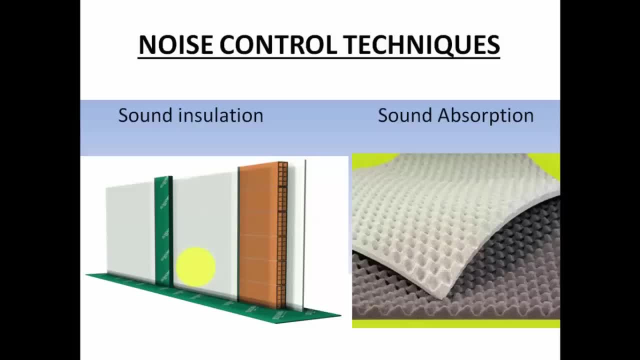 and success in achieving sound insulation actually depends on various factors. for example, what is the building structure, what kind of ceiling is used, what are the partitions, how big is the room. so all that actually will decide whether there is is proper sound insulation done or not, and how a successful sound insulation can be done for a proper building. 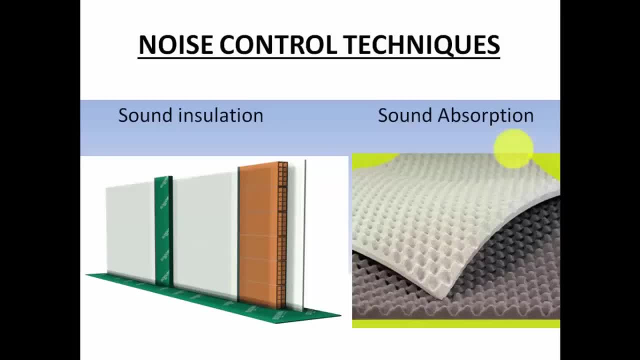 right. on the other hand, what is sound absorption? sound absorption means introducing some kind of absorbent material into the room so that, you know, the acoustic of the room can be altered in order to reduce the noise. that is called a sound absorption, right? so there is a very slight 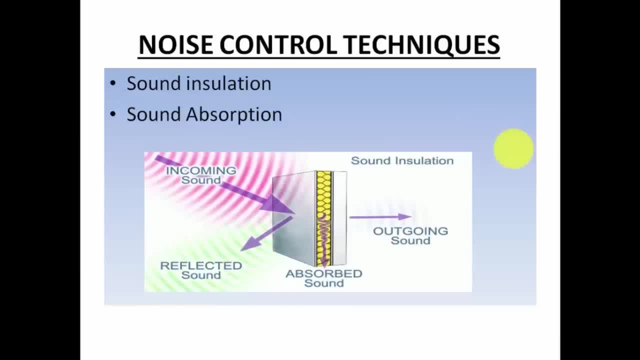 difference between the two kinds of techniques. now again, sound insulation and sound absorption. I have, uh, or with the help of a diagram I've shown here. so this is an absorbent material that is placed in between the two rooms, or let's say, in between two walls, so this will absorb sound. so 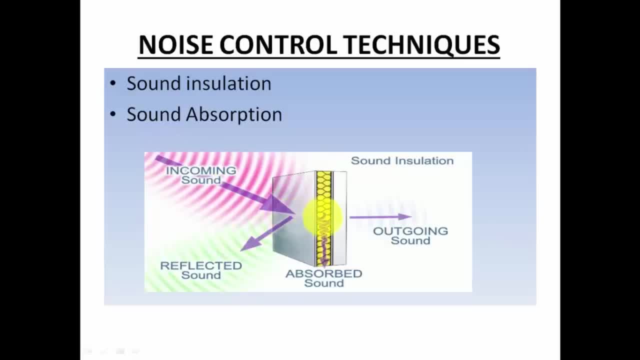 the incoming sound that is coming from here will be absorbed by this material, and the outgoing sound will be this. so, basically, the outgoing sound will be much lesser as compared to the incoming sound, whereas, on the other hand, this is sound insulation. right, sound insulation means the sound will. 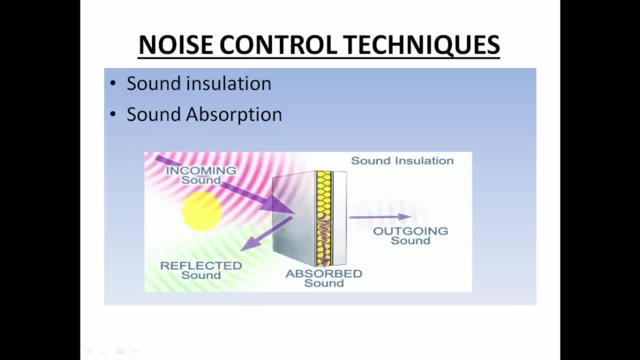 incoming is here, outgoing is here, but the sound will be reflected by this material. so this is sound insulation, right? so this is a reflected sound here. this is the absorbed sound. here both will be different and all these three will again be different. incoming sound will be much higher, the outgoing sound will be much lesser and the reflected sound 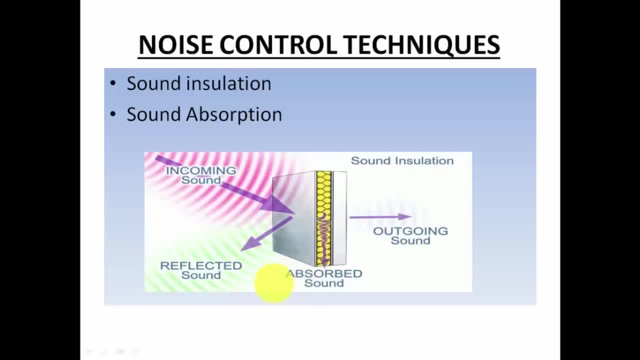 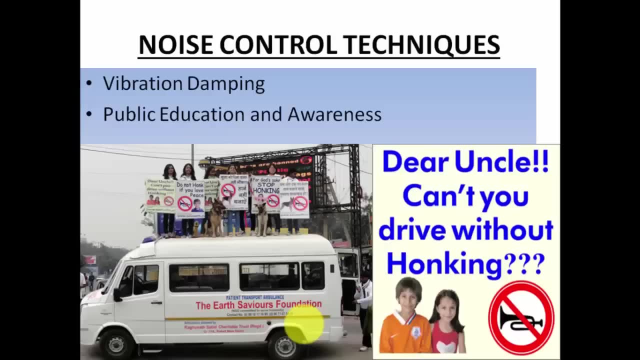 will be somewhere in between the incoming and the outgoing sound right. so this is what is known as sound insulation and sound absorption technique. now the other techniques of controlling the noise is vibration damping. vibration damping is a term that is used in as far as the industrial electronic 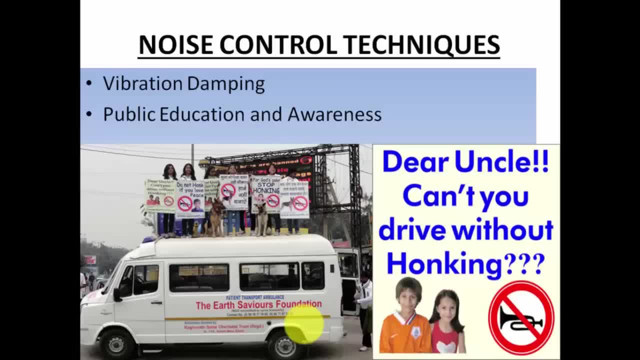 or ergonomic applications are concerned, where there is a need to reduce the amount of the energy that's produced by the system. vibration damping is basically reducing the vibrations. so if we reduce the vibration then the effect will be reduced. so if let's say we have an incoming 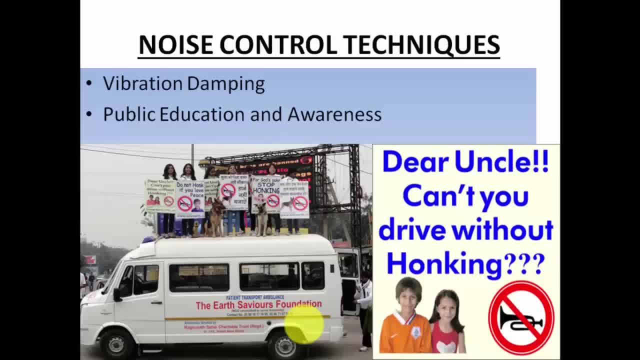 vibration. if vibration damping technique is used, the vibrations are reduced, so the outgoing vibrations will be, so the noise that is produced after vibration damping is done will be less, so this is another technique to reduce the vibration. lastly, and which is the most important, is public education. 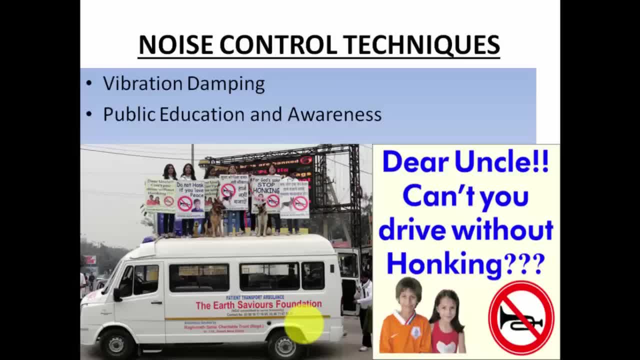 and awareness. what is required is that the public has to be aware of its ill effects. people has to be aware of the ill effects of sound pollution because, generally, what do we see? we see soil pollution because we see dirt. we see air pollution because we see the dirty air and the dirty sky. 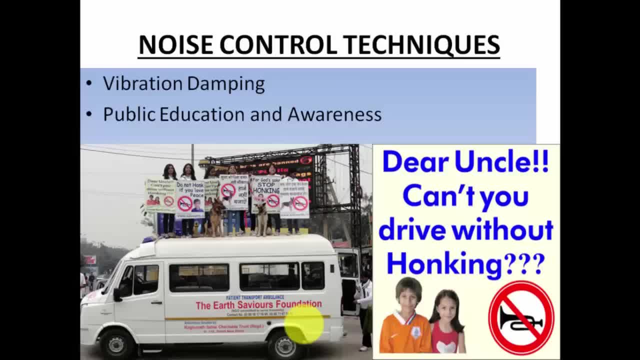 right, but we do. we see water pollution because we see lot of dirt and the dirty water being excreted out into the rivers, but we do not see noise pollution, because it exists for some time but the after-effects of noise pollution actually stays for long and it plays with the help or health of the human. 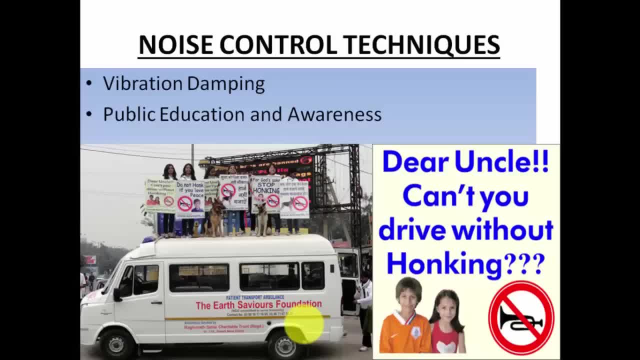 beings, health of the animals, health of the vegetation which is not visible. so that is the area that we have to control and we have to take seriously right. so these are the few noise control techniques by which we can control the noise pollution. also, let's learn about what does the law say is about noise? 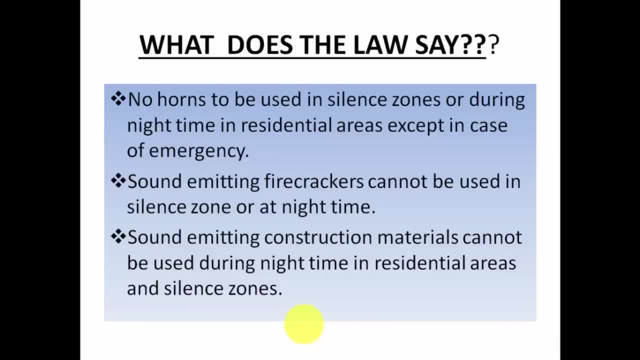 pollution. the law says that no haunts to be used in silent zone or during night times in the residential areas, except in the case of emergency. so this is a very major law which talks about unnecessary blowing of the horn. so unnecessary brewing of the horn during certain time is not allowed, right. 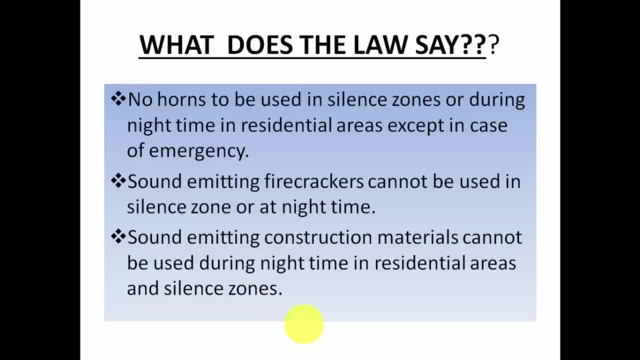 secondly, sound emitting firecrackers cannot be used in silent zone or at nighttime. thirdly, sound emitting construction material cannot be used during night time in residential areas and silent zone. here I have not discussed all the laws, because there are many other laws which exist as far as the noise pollution is concerned, but 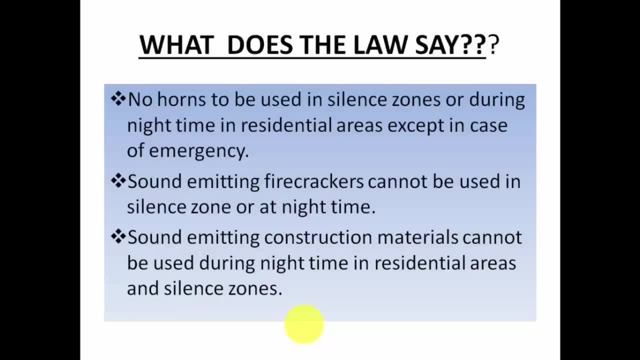 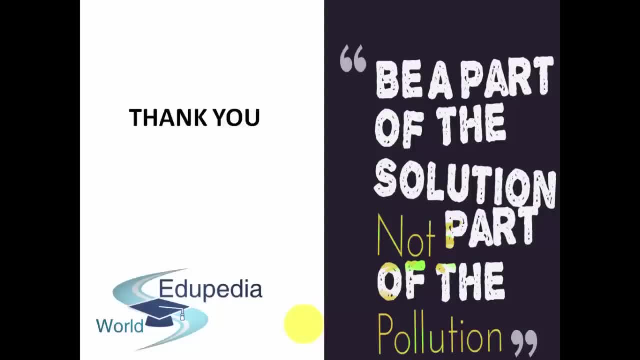 there are some laws that I have just flashed here. there are few other laws that exist. so now that we have gone through the entire tutorial about noise, noise pollution, the effects and the sources, and, finally, measures to control noise pollution- I hope it is- it is clear to you as to why. why is?